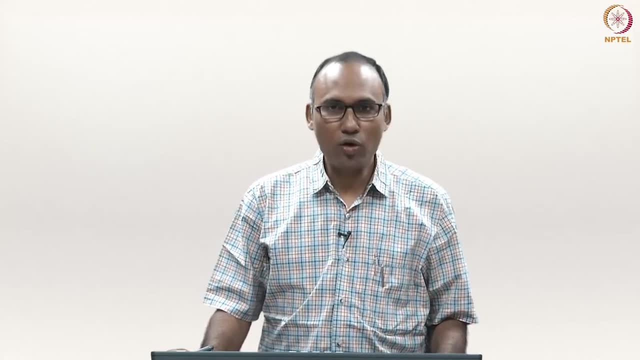 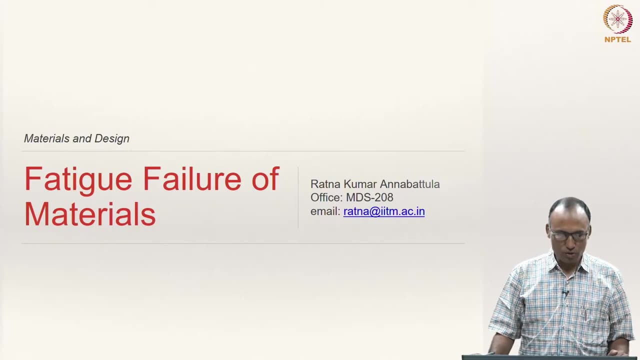 we have actually looked at static failure theories, wherein the load actually applied on the structure does not change with respect to time. all right, So now in this module we will be looking at fatigue failure of materials, which basically means the as a function of time, the load changes. So it is in other ways we could also call: 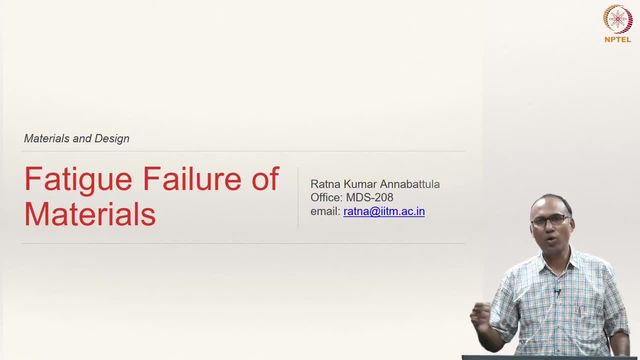 this as dynamic failure theories, because the load is changing, So the load is changing with respect to time and the and primarily when we are saying load with load is changing with respect, changing with respect to time. we are primarily interested in the kind of systems wherein load changes with respect to time in some periodic manner. 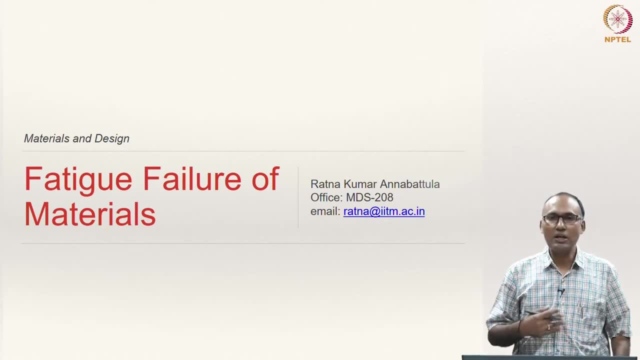 or a cyclic manner, And so that means there is a repeated load that is acting on the material, and such process is called fatigue. So the theories that we are going to talk about are called fatigue failure theories, and we will be spending some time understanding how fatigue failure happens and so on in this. 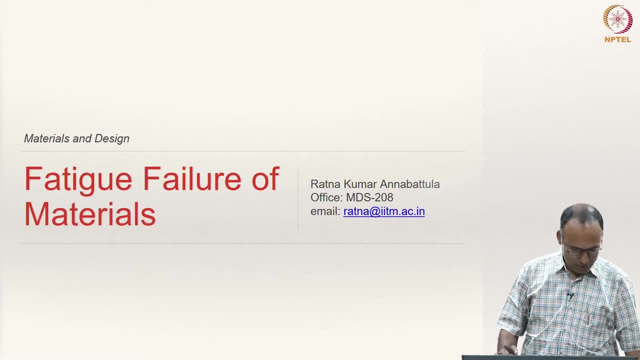 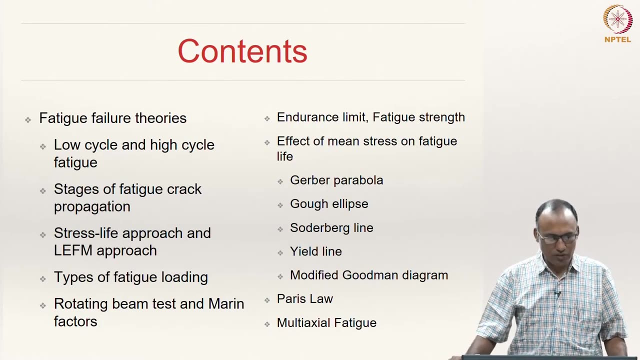 module. all right, So all right. So the contents of this module is basically: we will primarily introduce what do we mean by fatigue failure? and then we took a look at different failure theories and we also look at different kinds of fatigue loading, like low cycle fatigue. 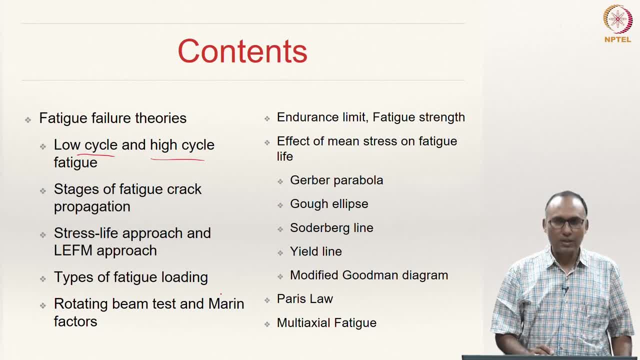 and high cycle fatigue. And then we will look at different stages of crack propagation under fatigue loading, or we call stages of fatigue crack propagation. And then we assess the failure of materials under repeated loading based on two approaches: one is stress, life approach, another and LEFM. 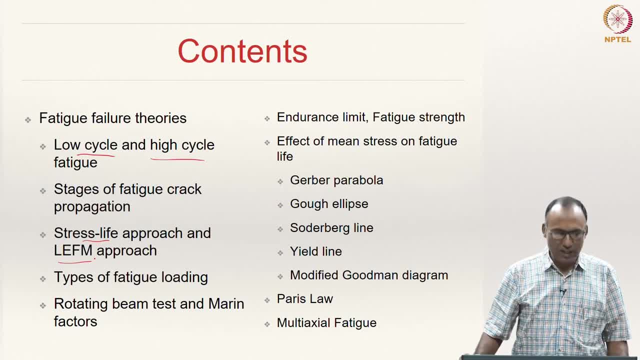 approach, or linear elastic fracture mechanics approach, wherein we do not consider any plasticity whatsoever. all right, And then we will look. we will also discuss what are the different kinds of fatigue loading and we will also spend some time on understanding a very important experiment that actually 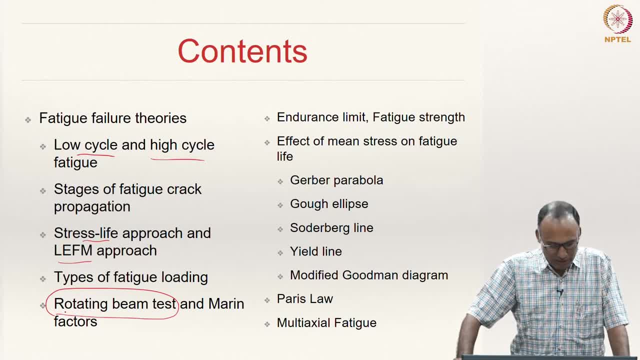 gives us some understanding about fatigue failure and such that experiment is called rotating beam bending test, And then we will talk about some failure factors that needs to be taken into account, depending on various conditions, are. they are called marine factors, And we will discuss what is endurance limit and what do we mean by fatigue strength and 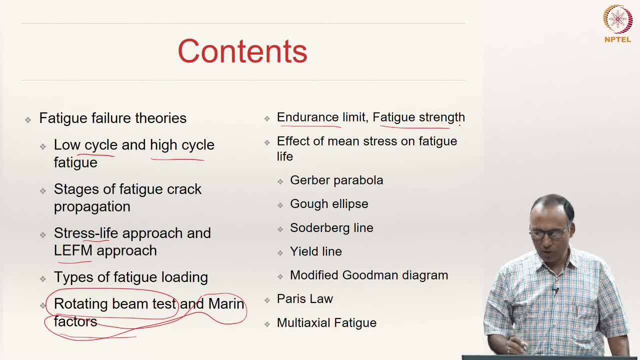 then we will spend a little bit of time on understanding what is the effect of mean stress. it will become clear when we get there. But then the effect of mean stress. based on the effect of mean stress, we would define different kinds of failure theories, such as Goodman diagram. 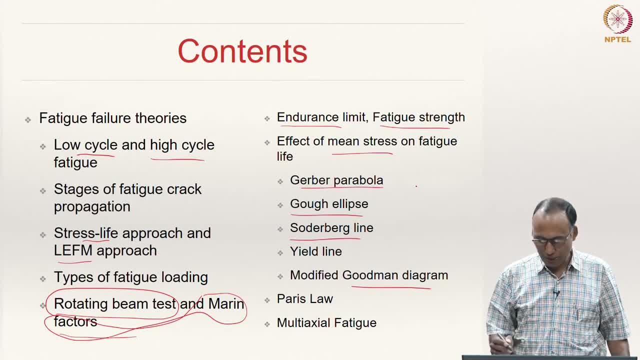 Soderbergh line, Babylobes, Gerber, parabola and so on. All these are different kinds of failure theories that take into a account of the presence of mean stress on the material, all right, And then we will look at the crack: life or fatigue. 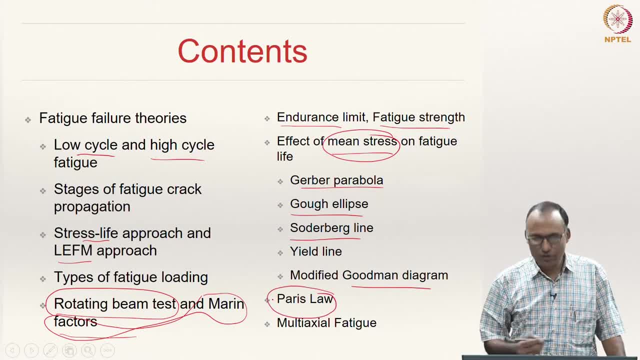 crack propagation as derived by Paul Paris on informal child's production. In this З and which is famously known as Paris law, We will spend some time on understanding crack growth rate in some sense, and then we will briefly introduce how do we go about dealing with multiaxial fitting, because until just before this module, this topic, we will be primarily 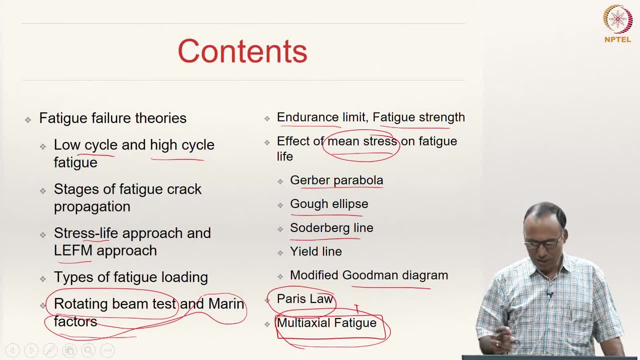 focusing on uniaxial loading. That means the loading is. so. if you are looking into from the concept of stress tensor, we are actually looking at the existence of only one stress component, such as sigma xx or sigma yy or sigma zz. not all, three or two are present. 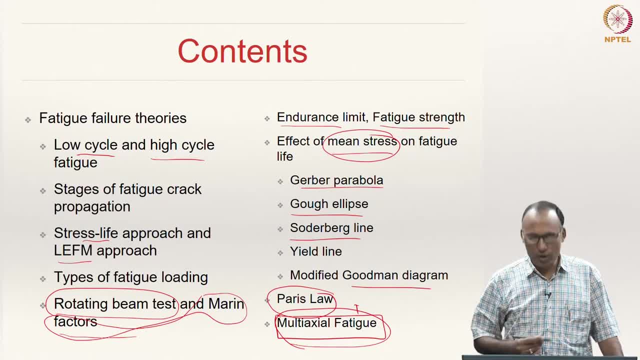 only one component is present. The moment you have a multiaxial loading, you actually need to develop a separate theory for multiaxial fitting, similar to what we have done in the static failure theories, wherein we have discussed some something called von Mises. 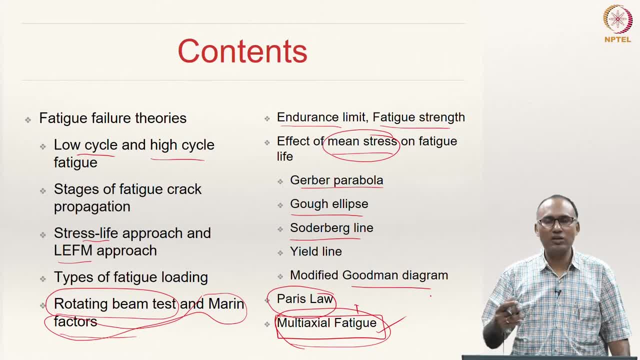 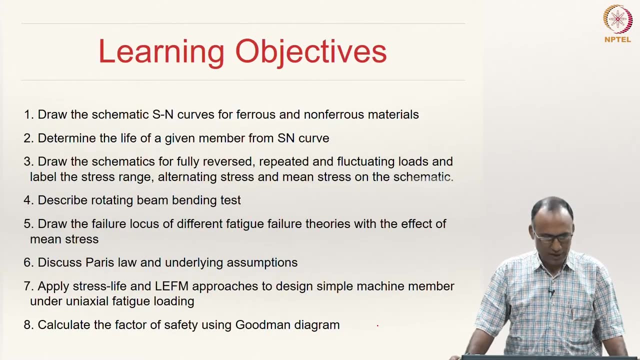 This theory wherein you actually define something, something called equivalent stress, which is an one dimensional equivalent of a real 3D state of stress. A similar discussion we will have when we are going to discuss about multiaxial fitting. So these are the learning objectives. 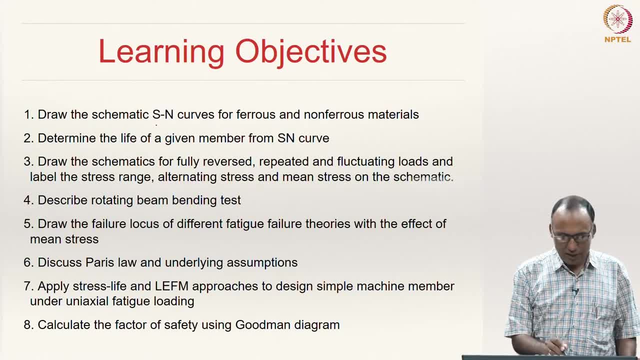 So we should be able to draw the schematic of S n diagram or S n curves for both ferrous as well as non-ferrous metals. So we will see what is the difference when we are going to the room. So we should be able to draw the schematic through the material, and we need to, we should. 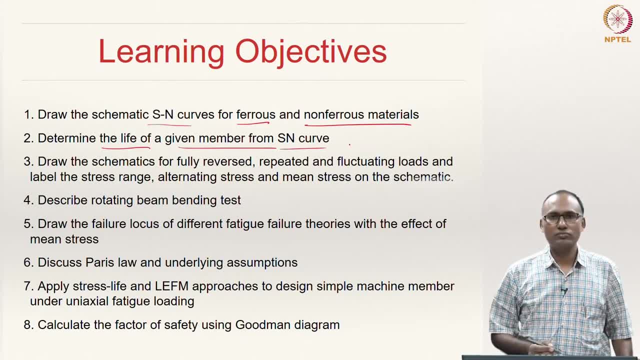 be able to determine the life of a given member from S? n curve. So you given if by knowing the S n curve and if you are know, if you know what is the loading scenario, then you should be able to predict what is the life of the component. that means how many, how much time. 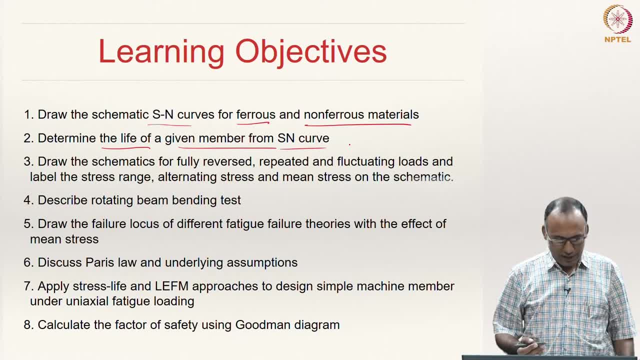 can you use this component at that particular load level, And then you should be able to draw the schematics for different kinds of fatigue loading, such as fully reversed, repeated and fluctuating loads, And you should be able to lay the stress range- alternating stress and mean stress- on the schematic. 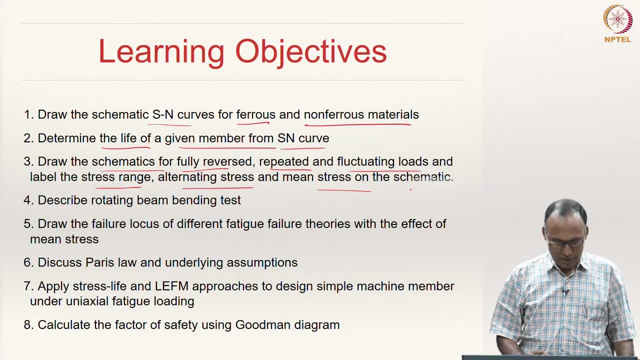 And, as I have already mentioned, one of the most important experiments in understanding fatigue life of materials is rotating beam bending test, and we will see how the test is conducted and so on. And then we will focus on drawing failure locus for different fatigue failure theories with the effect of mean stress. that means until here we will assume that 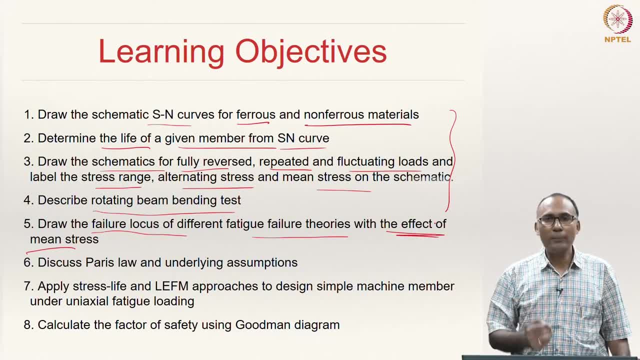 there is no mean stress, stress. And now, if there is mean stress, if the mean stress is 0, what happens is what we will study first, And then, if we have a non-zero mean stress, what happens is will be will be studied in this module, And then we will try to draw the failure locus for. 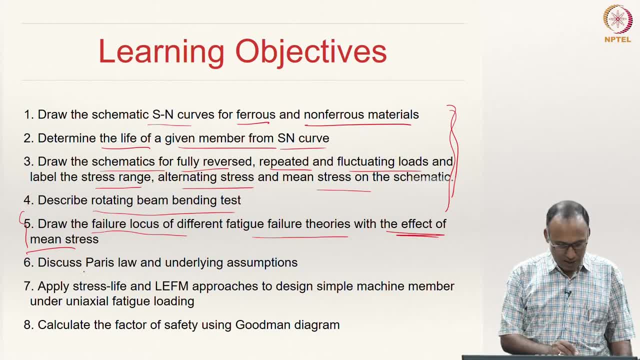 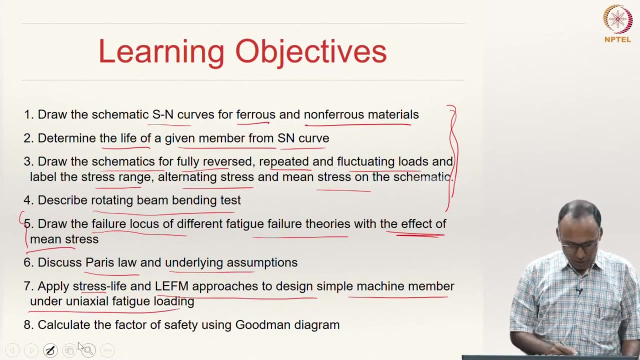 each of these different failure theories And then we will discuss Paris law and the underlying assumptions And then the apply stress, life and LEFM approaches to design simple machine members under uniaxial fatigue loading ok, And then we will also be able. 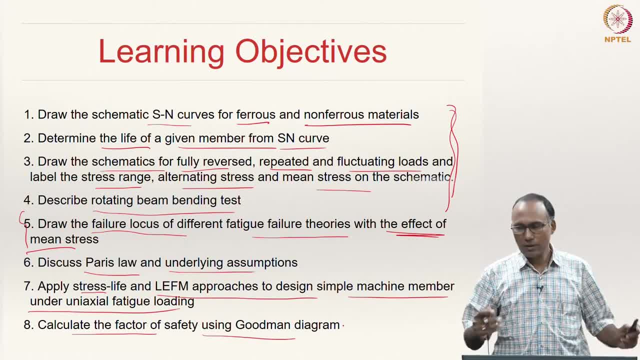 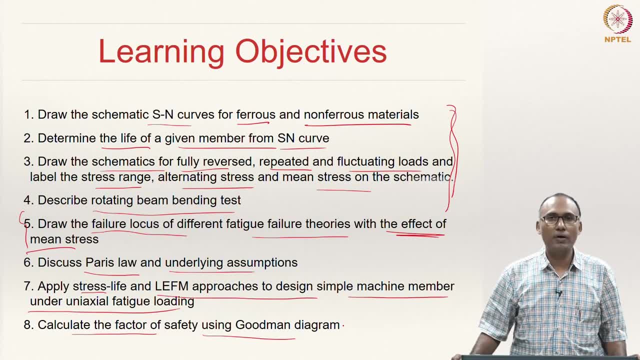 to calculate the factor of safety using Goodman diagram. So, like the way that we have done the calculation of factor of safety for, for instance, von Mises theory or distortion energy theory or maximum shear stress theory, You have drawn the diagram and then, if you are able to identify the stress state, then graphically, we were able to find: 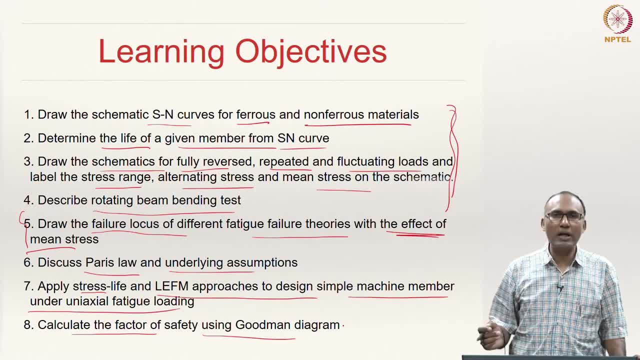 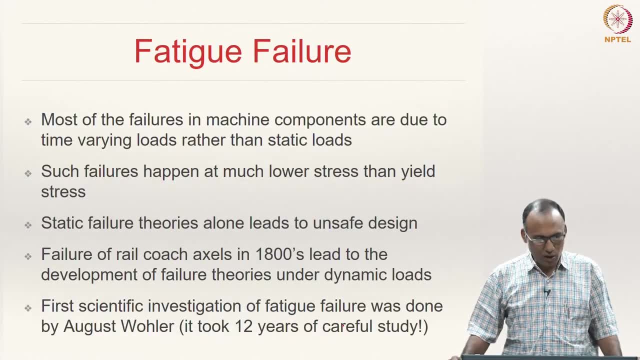 out. what is the factor of safety? Similarly, on Goodman diagram, if you are able to identify the stress state and then you should be able to calculate the factor of safety, all right. So what is fatigue failure? So most of the failures that we see in machine components. 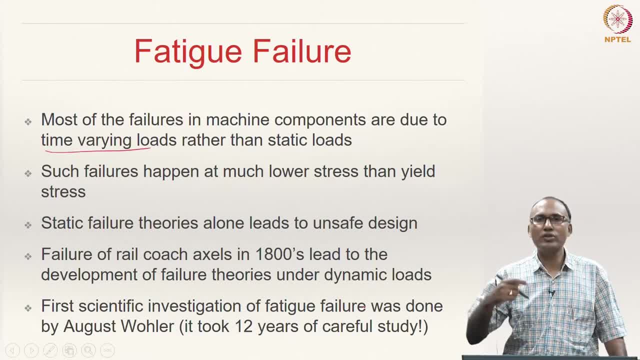 are due to time varying loads right. Suppose, if you take a shaft right transmitting power and you let us focus our, So let us say: this is our shaft, It has a kg and it is rotating along this axis, And then it is rotating about this praxis. 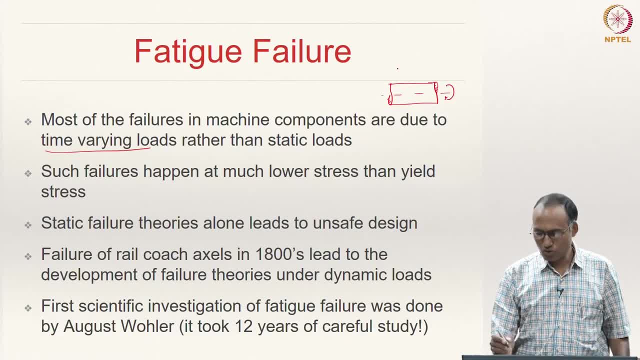 right, And then it is rotating about this axis and then transmitting power. there is a gear sitting on it, and so on. And then let us focus our attention to this element and let us say there is a gear sitting on it, So, and hence, as a result, the shaft 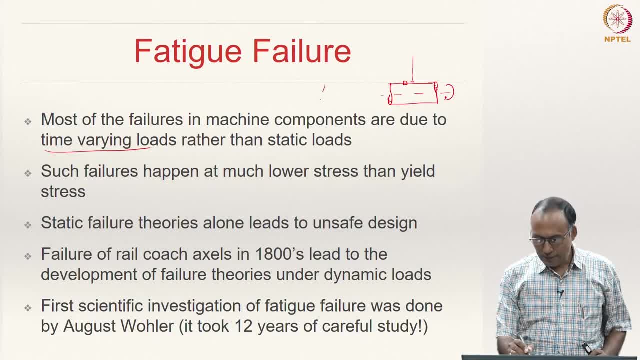 bends and then it rotates. And when the shaft is bending like this, we know that there are going to be compressive, there is going to be a compressive state of stress on this layer and tensile state of stress on that layer, But the fact that the shaft is rotating, so 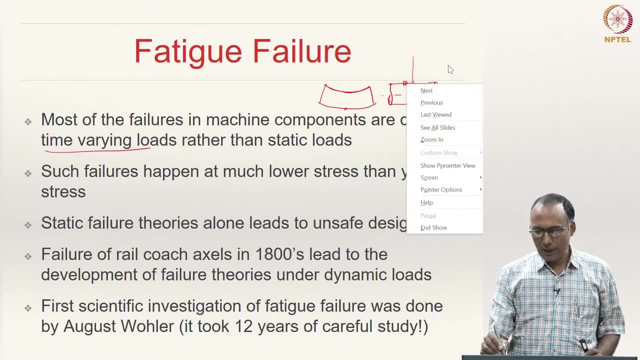 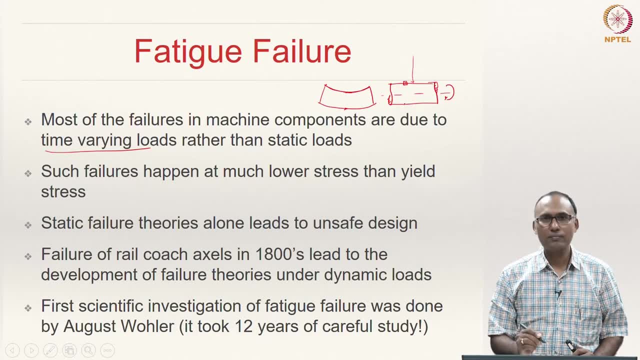 the point which is on the top to begin with by half a rotation. by the time it makes half rotation, then what happens? this point will move here right And initially the point which is at the top, because always the load is not changing the position. the load is there and this point was initially in the state of compression. 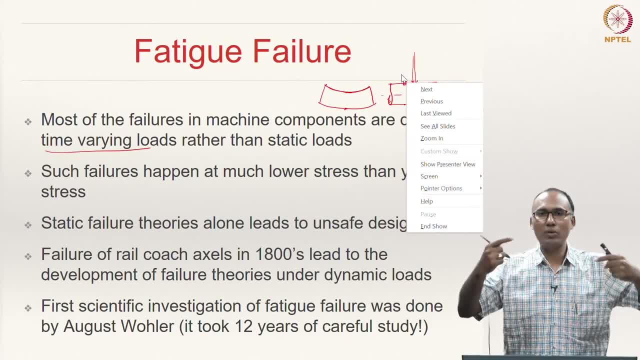 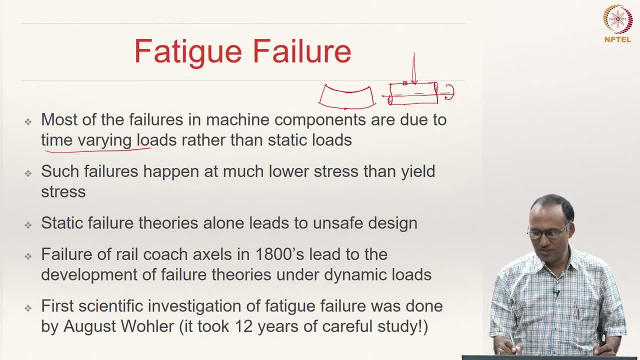 but when it makes one half a rotation, the state of stress changes from compression to tension, right And since the stress, the diameter. this is a symmetric about this axis and hence the magnitude of the tension and compression will be the same. that is something that we have learnt in our strength of materials class. And then what happened? what is happening here? 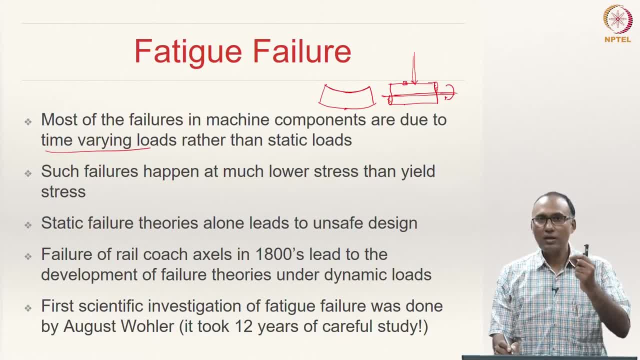 is that the same material point is changing. it is a stress state And ever the same, the action is happening here, right? So if we count this component space as a maximum point which is included by number of del square right And the less theありがとうございます inside the d campus, it means we are going to put same 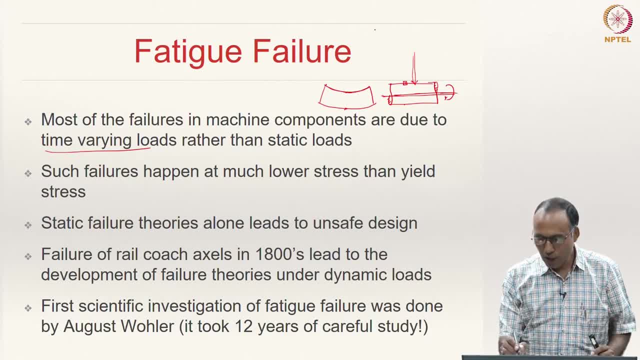 value in between the d plus del square right, and so the very great value occurring here in the sediment at each point, the entire mass Ч개� B, América B, in every point, while theosaic mass is going from compressive to tensile in half a rotation and then making 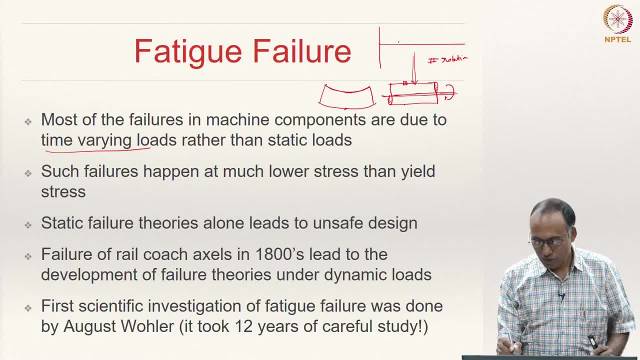 a full rotation, it will go back to the compression again. So if you we could draw, let us say, number of rotations on the X axis. So one rotation 2, rotation 3, rotation, 4 rotations and this is my half rotation. So this element initially. 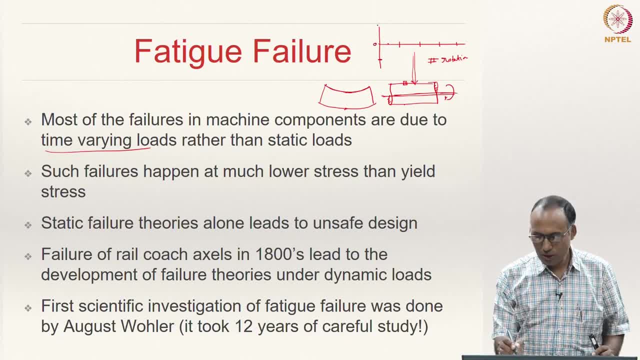 is having the say. let us say some compressive stress. this is 0 and let us say the magnitude, magnitude equal, and my equal magnitude is tension. let us say: this is my sigma and this is also sigma. this is negative sigma, that is positive sigma, all right. 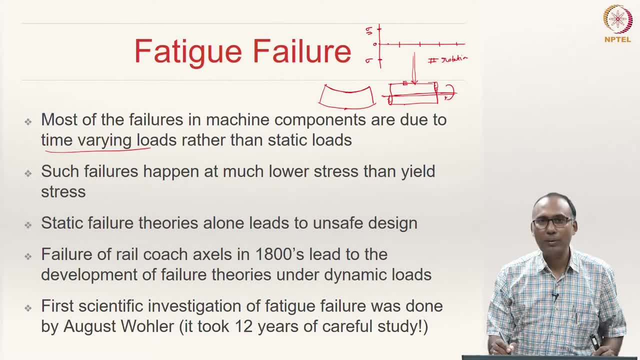 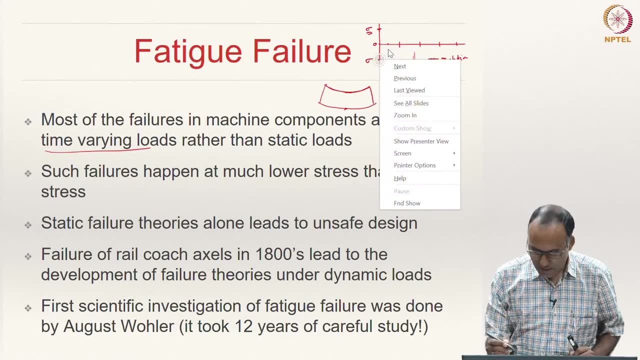 And now, initially at in the beginning, when the shaft is about to start, at the first rotation, the stress is this: and by the time it makes half a rotation, it the stress state is going to negative, positive. So this has become like that, all right. And then when it will, 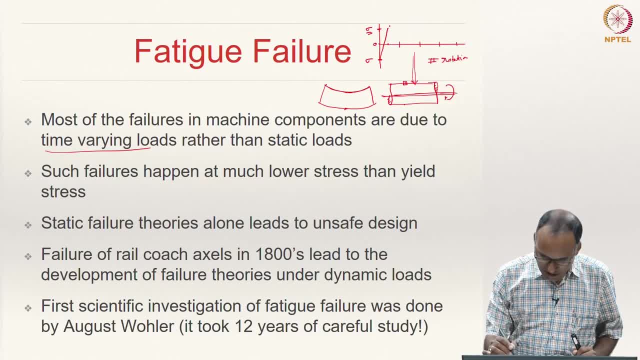 make full rotation again, the stress state- sorry- will become negative again, and so on. It continues to do so. so because for one rotation, within one rotation, it has come back to its original configuration, but during this time, the material point has changed its stress state. 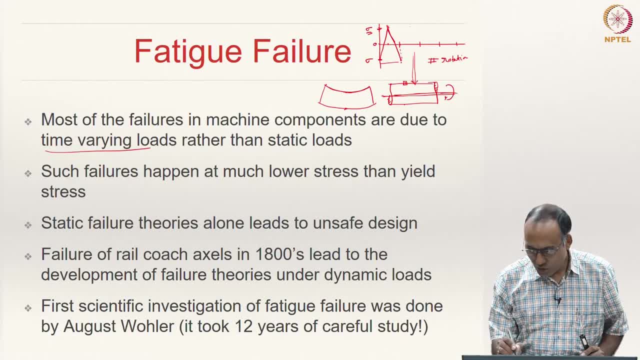 And if you continue this again and again, so you will have the material point- keeps on experiencing this variable stress: positive, negative, positive, negative and so on. right, That means at a given point, the stress state is changing with respect to time, That means the load is getting repeated and 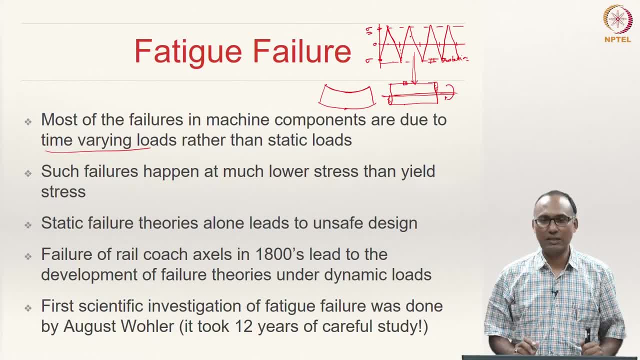 such a process is called fatigue. ok, So, as we know, most of the material machine components are subjected to this kind of time varying loads rather than static loads. right, Most of the machine components that we are deal, we deal with day in and day out, are subjected to this kind of fatigue load. For, 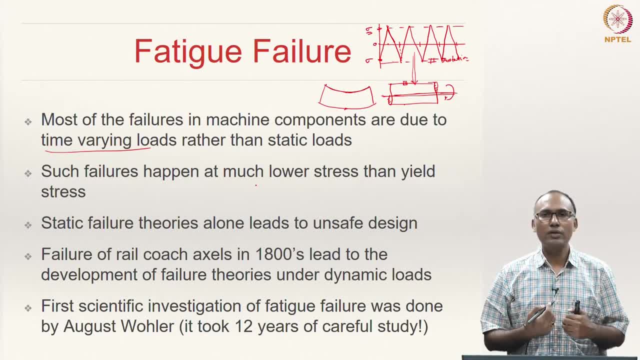 instance, if you take your cycle bicycle and then the the sprocket teeth on the bicycle are subject to to fatigue failure because at a point the number of sprockets teeth that are contact in that are in contact with the chain or less than the total number of sprocket teeth. 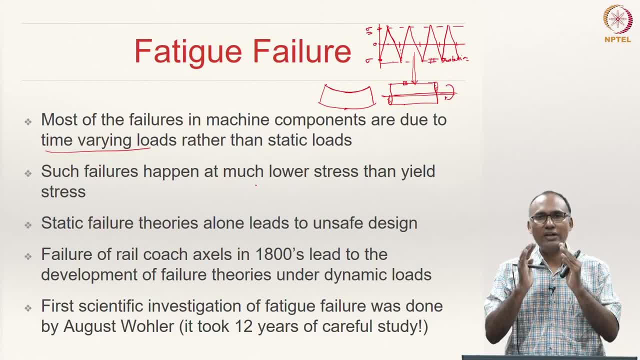 And hence some of the teeth are having a finite amount of time in one particular rotation, one rotation completely. it will not be in contact only sometime right During the time that it is not in contact, the force exerted on to the sprocket teeth is actually 0. That. 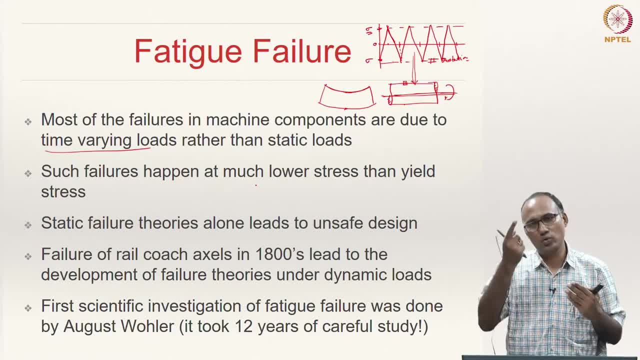 means your load is varying from some finite load to 0 and so on. it is cycling between these two. So like that, you can take several examples, and most of the systems are subjected to time varying loads And when sub, it is observed that when such systems, when you, the 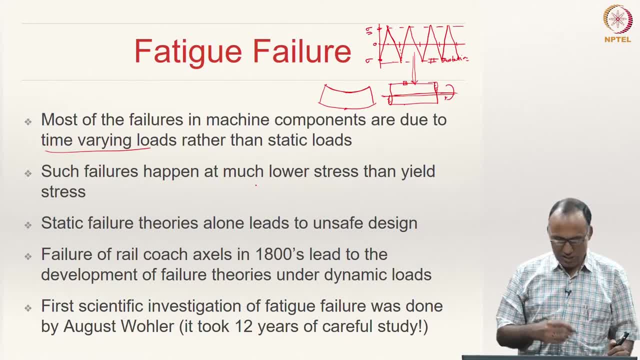 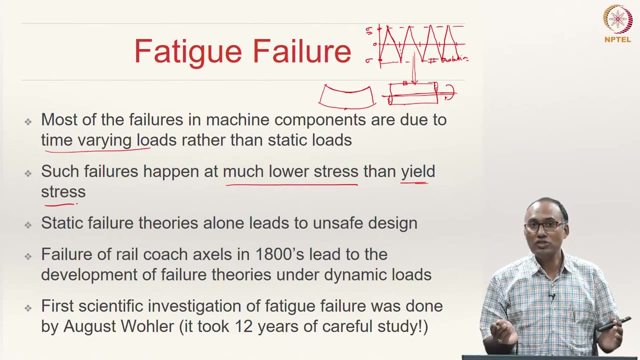 systems are subjected to this high- This time varying- loads, it is observed that whenever they fail, they actually fail at much lower stress than the yield stress of the material. But when here we are saying, when we say fail, they are actually breaking, It is not like the ductile failure that we are. 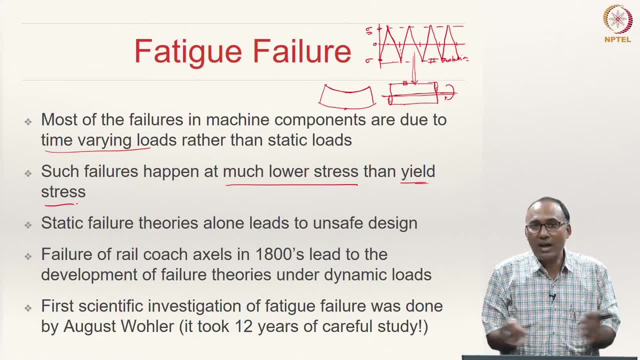 talking about. it is actually we are talking about a fracture, like in a brittle manner, But there may be some local plasticity, but we are actually talking about failure in a forget. the failure is actually happening much below the yield strength, which is not what we expect from the perspective of static failure. 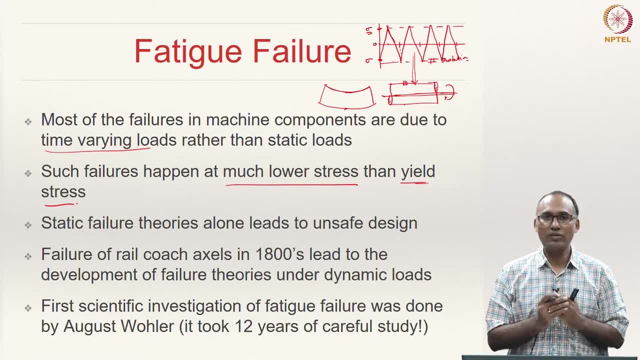 But in we can the case of fatigue failure or when there machine member is subjected to time varying loads, we see that the materials are actually failing much below their yield strength. So people were, or not, puzzled about this particular strange phenomena, while we know that the material does not vary than 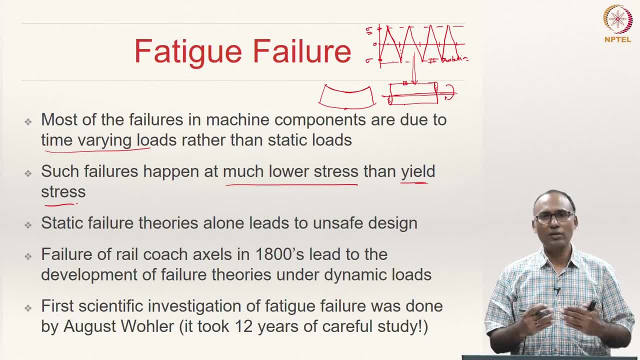 go beyond ultimate when you are talking about yield strength. that material does not enter plasticity below the yield strength, but when the load is changing with respect to time, people have been observing that the material is actually failing below the yield strength right. So that means you cannot explain this phenomena based on the lessons that we. 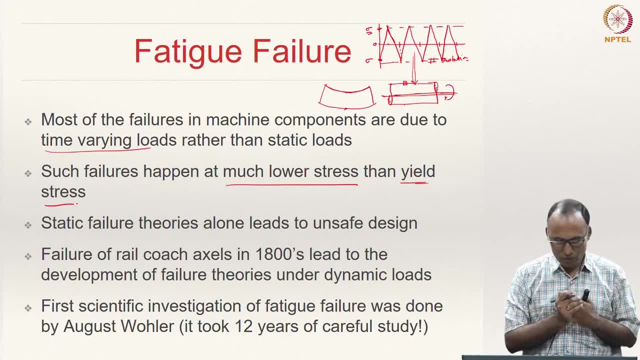 have learnt until now based on the static failure phase. So static failure theories alone leads to unsafe design, because we people have been observing that the materials are failing when the service load is actually below the yield strength of the material. ok, So there are in in the history. there are several cases. 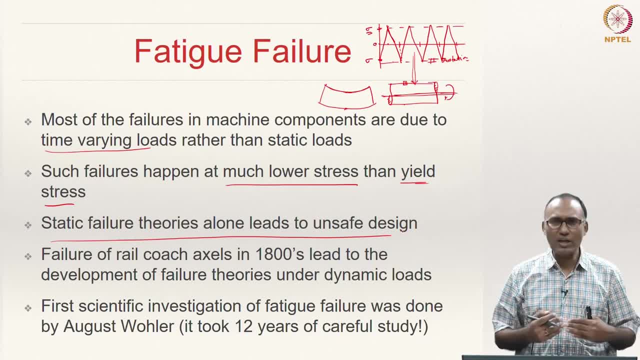 where people, there were several casualties, just because the designs were not taking into account of this nature of time, varying nature of the load, which actually led to failure, premature failure of the components than the what engineers thought those days will withstand right. So, for instance, the failure of rail coach axles in 1800s led to the development. 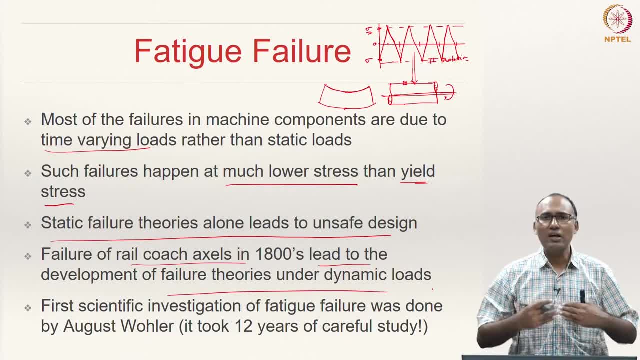 of failure theories under dynamic loads. The several railroad accidents around 1800s, both in Britain and Germany and then that led people to pay attention, to understand this particular phenomena and that is what led to the development of failure theories under time, varying loads. The first ever scientific investigation, a detailed scientific scientific investigation. 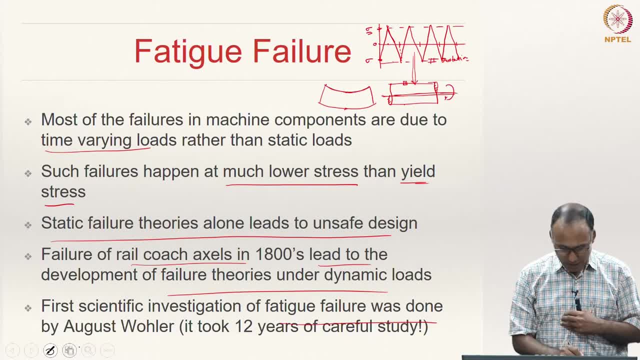 of fatigue failure was done by August Wuhler in Germany, where he spent almost 20 years of his life understanding, doing several experiments and trying to understand what happens when you subject an axle to a repeated load, and then how does the material fail? It took his 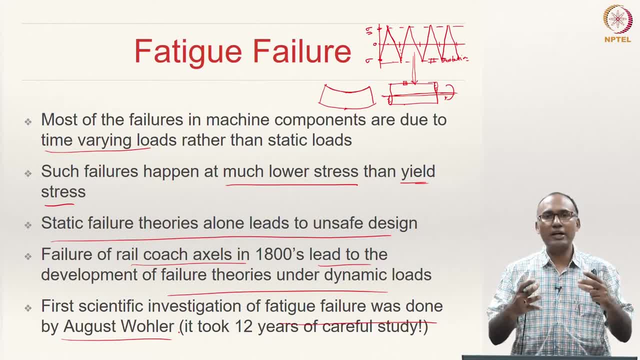 him 20 years To consolidate his experimental data and write one single paper. but that happens to be the seminal paper in the literature of fatigue failure and till date people ah refer to that work because of the impact that work had on the design or the or the design philosophy. 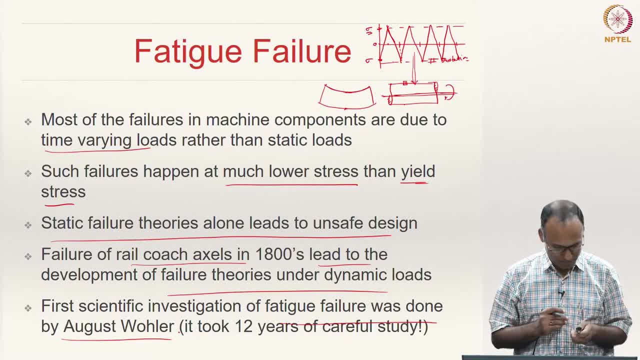 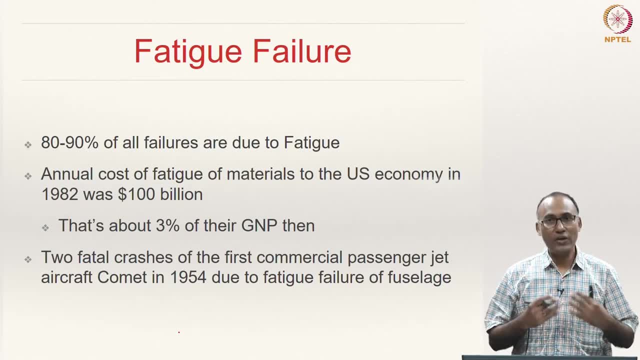 of machine components that are subjected to time, varying loads. alright. Then you actually look at several failures, failures and when. for instance, when you do post mortem of several industrial failures, it turns out that about 80 to 90 percent of all failures are due to fatigue, and such is. 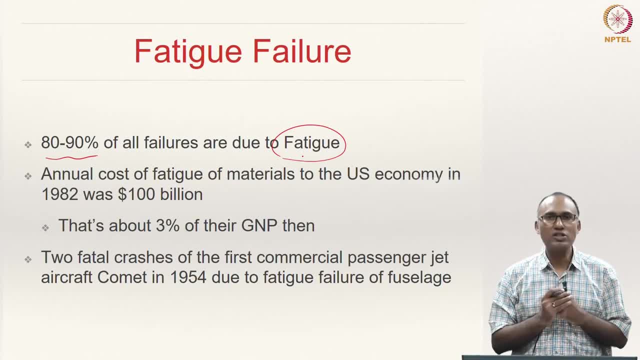 the importance of understanding this particular field of failure, the fatigue failure. The annual cost of fatigue failure, fatigue of materials- to the US economy in 1980s was about 100 billion dollars. that is about 3 percent of their GDP. So there are several. 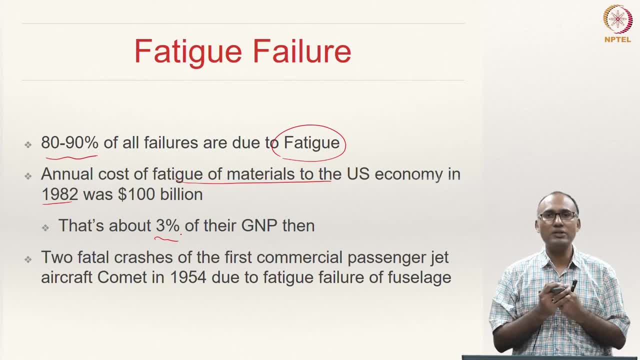 countries which actually spend much less than 1 percent of their GDP on the entire science and technology budget. but the cost of fatigue failure alone in 1980s was about 3 percent of the GDP of United States. And you can imagine what if you neglect this particular field of failure: understanding of the failure of this kind. 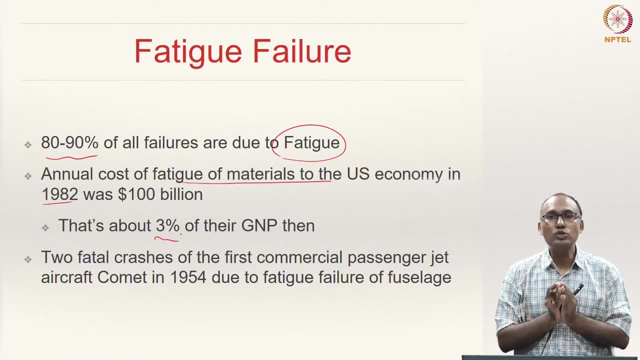 of systems, what kind of a catastrophe that it can lead to the economy. And one of the very sad stories primarily about aircraft industry is on the comet aircraft. There are two fatal crashes of this first commercial passenger jet right in 1954 happened due to fatigue, failure of this And 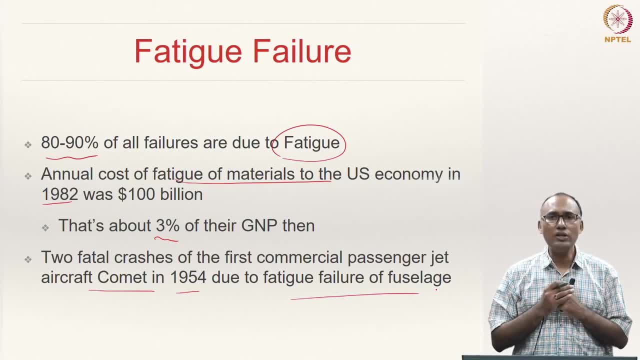 there were some design issues which led to such a fatigue failure and that actually led to bringing down the entire fleet of comet and, as a result, they lost their market to their competitors elsewhere in the Europe and in the US. So this is a very sad story. 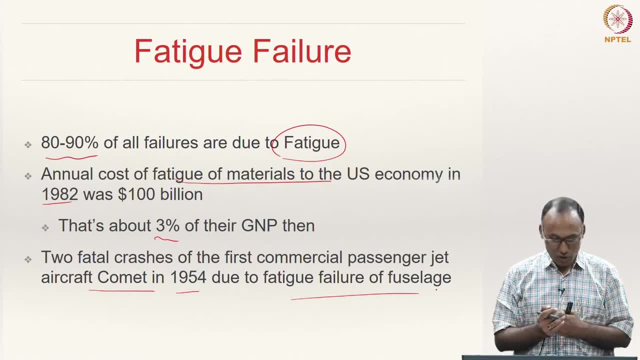 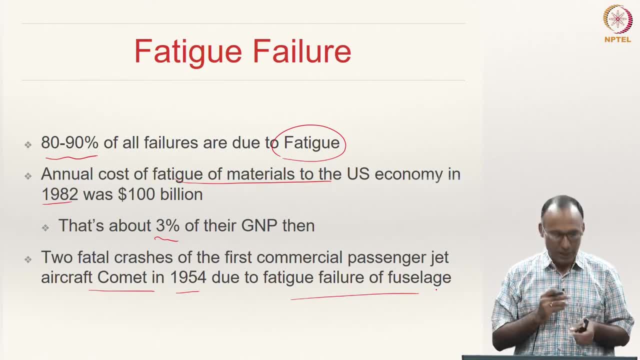 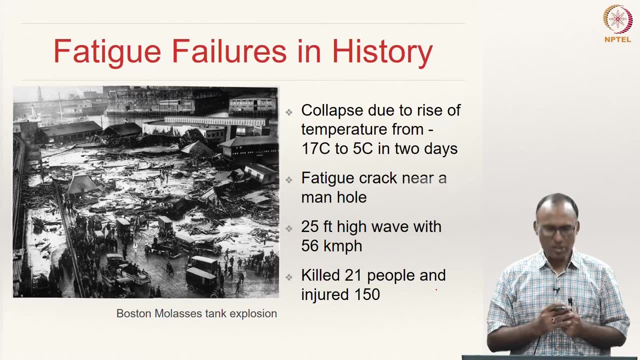 can bring down economies significantly if you do not pay enough attention. So let us spend some time on fatigue failures in history just to understand, just to put things in perspective and try to understand what is the magnitude of fatigue failure and USA. So this whole topic currently is being 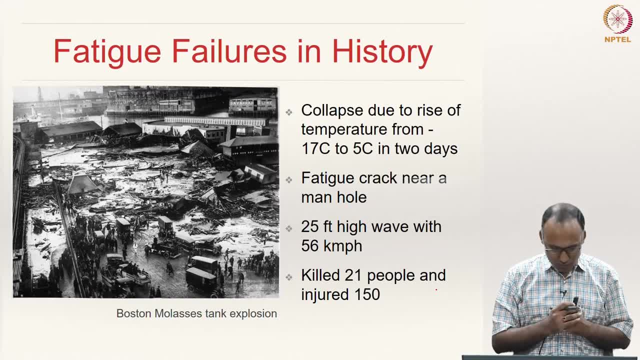 discussed as it is highly prestigious. So this opportunity is by no means recommended. the United States does not mean much when it comes to所 downforce and such that really enjoy the such a failure. So this is a famous Boston molasses tank explosion. So this explosion, 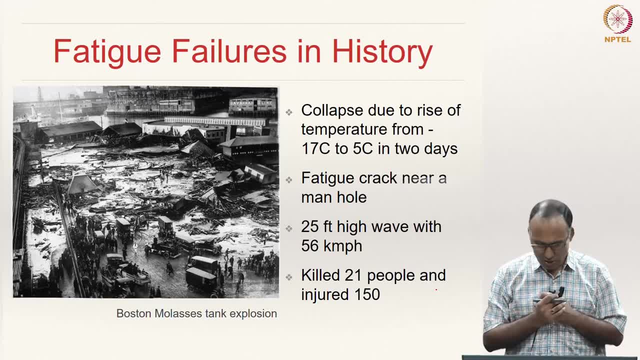 there was a molasses tank in the city of Boston and one early morning, suddenly this molasses tank exploded And then, if you see this, there are so much of wreckage around here and about 21 people killed, almost 150 people got injured in this accident. And the reason for and then 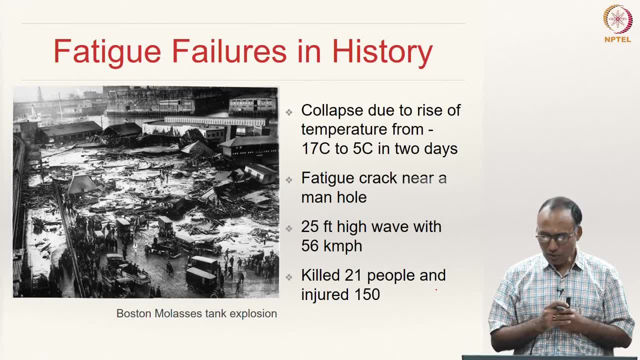 the people looked at what could be the reason and they figured out that it the collapse happened due to rise of temperature from minus 17 degree Celsius to 5 degree Celsius in 2 days. It is about a temperature rise of delta T of 22 degree Celsius and, as I mentioned, 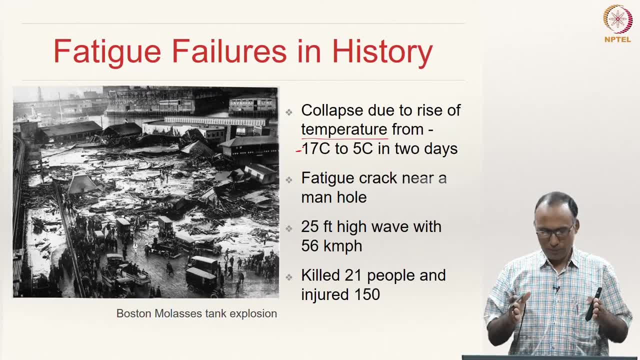 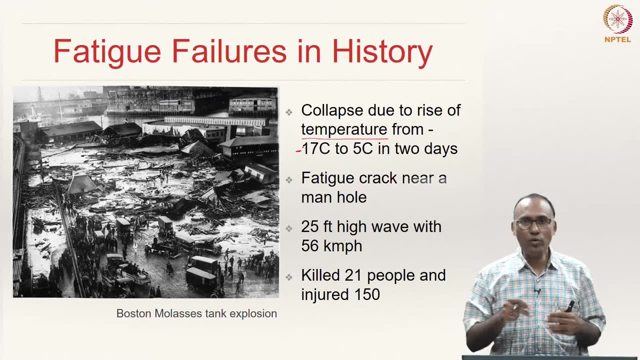 the result: within 2 days, you have a this temperature gradient and that actually led to the failure. How? Because in on the manhole, one of the manholes of this molasses tank, there was a fatigue crack that developed because of this change in temperatures. When you are, 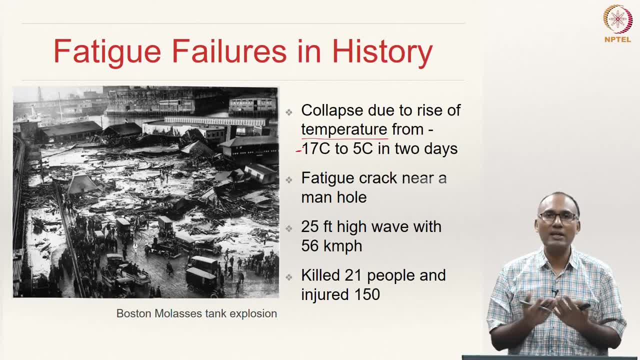 having change in temperatures. what, basically, what we are talking about is the time varying load, right, So the thermal stress is cycling and near a manhole, which is a stress concentration, a crack got initiated and then that crack became critical crack during these 2 days. 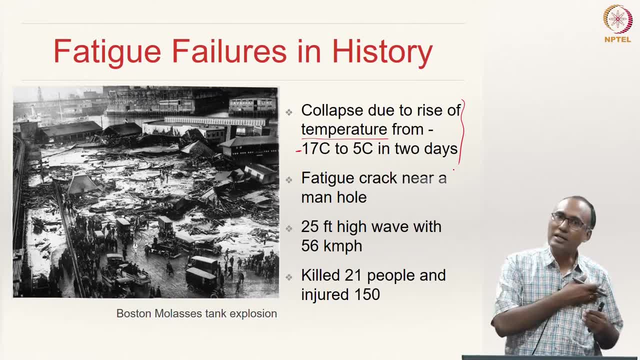 of delta T variation, temperature variation, and then suddenly it broke like a brittle fracture and the molasses tank broke apart And, as a result, whatever is the material, the molasses is a viscous liquid and when it broke it was like it led to a 25 feet. 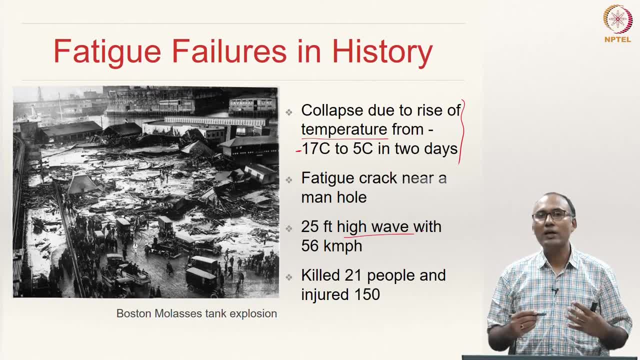 high wave of molasses, So there is a high viscosity of molasses, going at 56 kilometers per hour. right, So it is not like a regular water, but it is highly viscous liquid and then once somebody traps, once somebody gets trapped, it is extremely difficult for them to get out, right, because 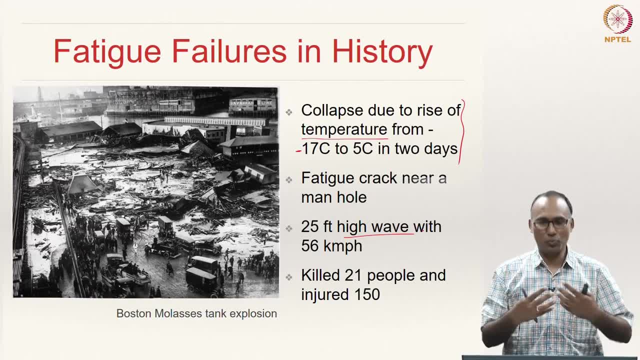 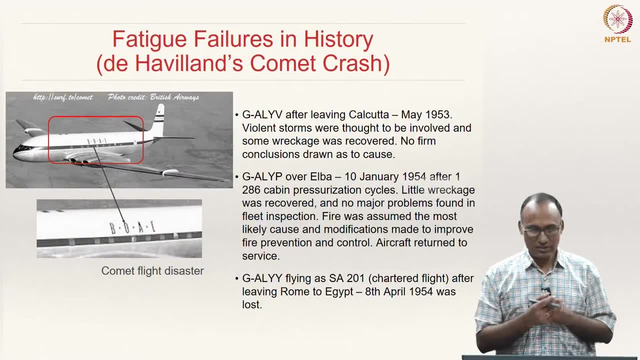 of the high viscosity you cannot even swim or move through right. It led to killing of 21 people. Another, as I was mentioning, comet crash. this is one of the most important thing: sad stories in the aircraft industry, wherein. So there are actually couple of accidents. 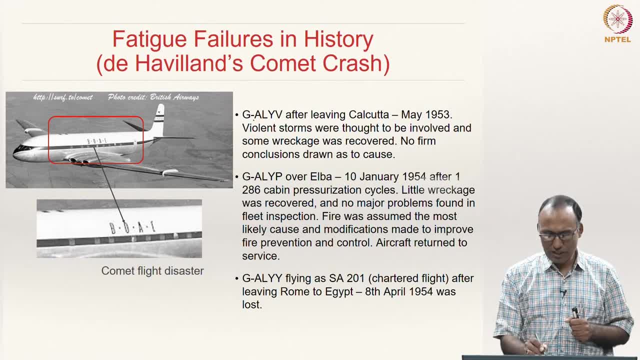 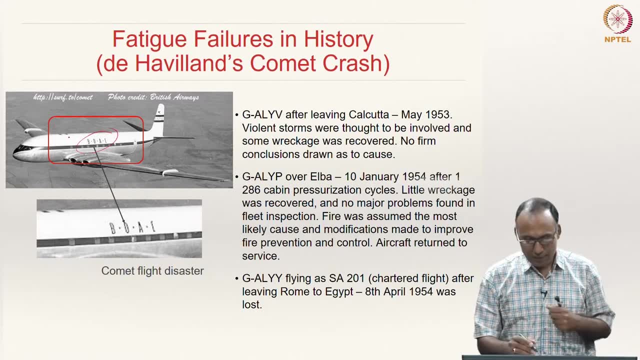 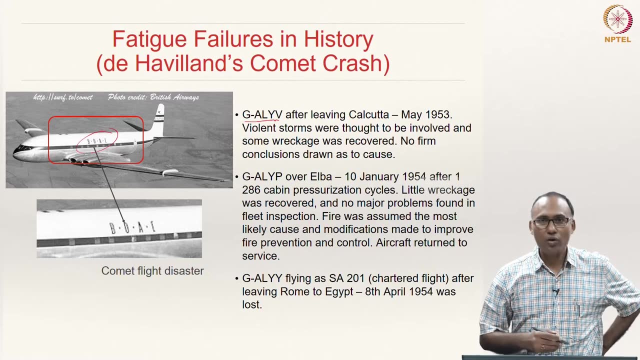 one after the other. So the first aircraft GA. it is managed by BOAC British Overseas Aircraft Company and the first model of their aircraft called GALYV. So it left Kolkata in May 1953 and then midway the flight got lost and people thought there were violent. 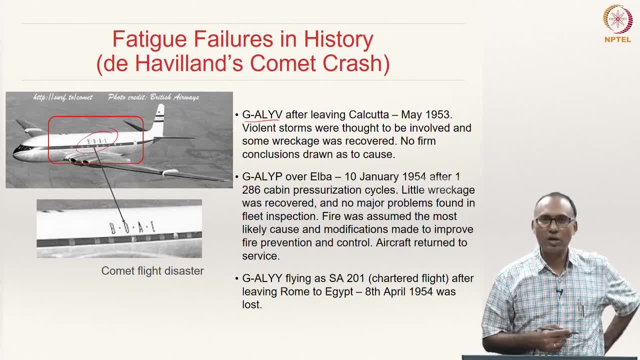 storms during that time and hence people thought the violent storm was the reason for the failure of this particular flight. and later people in recovered some wreckage and but they could not draw from conclusions. And then again, almost 6 months or 7 months later, they had next model GALYP, and on 10th. 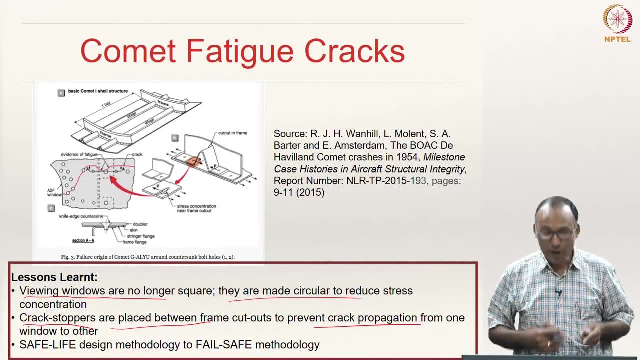 So that is what is called fail safe design, and then now today's aircrafts are actually following fail safe design methodology. So you can see, the one sad crash actually led to several new consequences and several consequences and several development of complete set of new design methodologies for the entire industry. 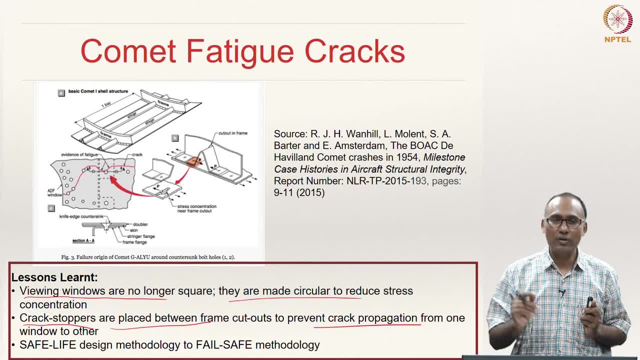 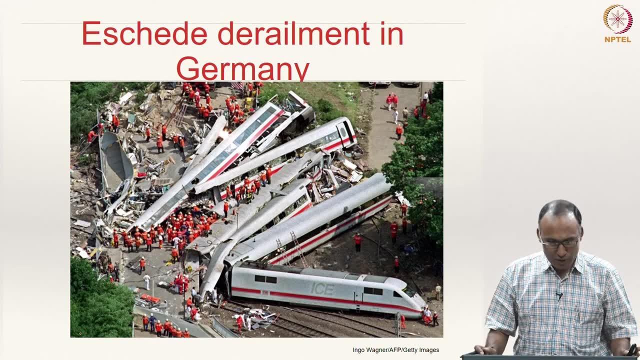 And there is any very important lesson that was learned from the sad story of comet. So the other sad accident in the history of German railways is issued, a derailment in Germany. So Germans high speed trains or ICEs – Intercity Expresses are known. 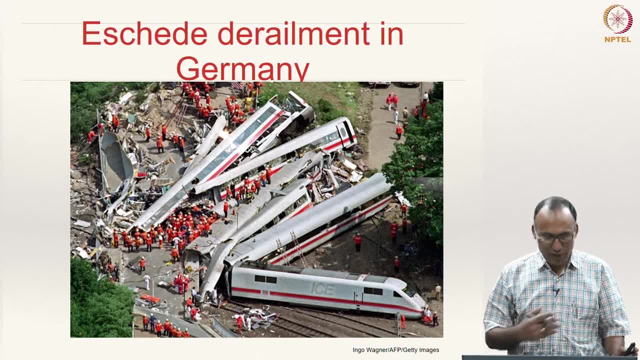 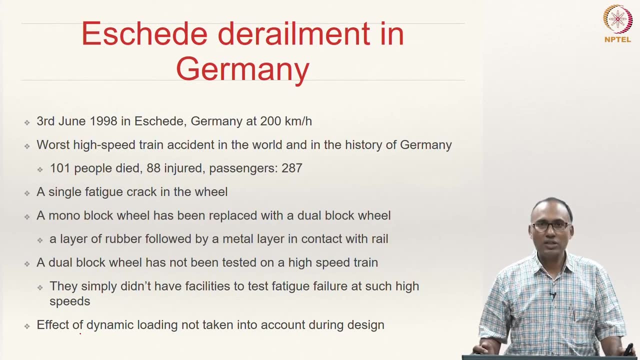 to be really high, very good high speed trains in Eiltsch in Europe, and they are known to be very efficient in their operation as well. However, in 1998, on 3rd June, the German Railway, or Deutsche Bahn, had a very sad accident at Isiede, famously. 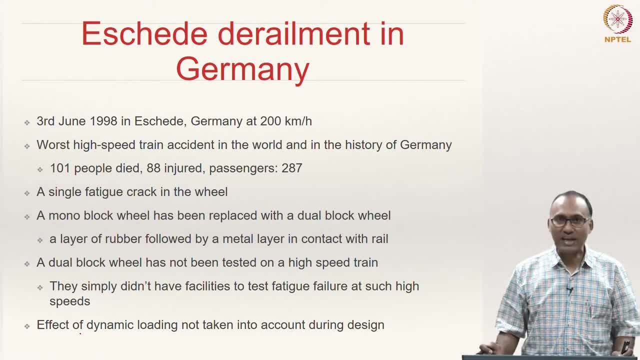 known as Isiede derailment, when this ICE was going at 200 kilometers per hour And during this time. this is possibly the worst train accident, high speed train accident in the world and also in the history of Germany, because this led to the death of almost 100. 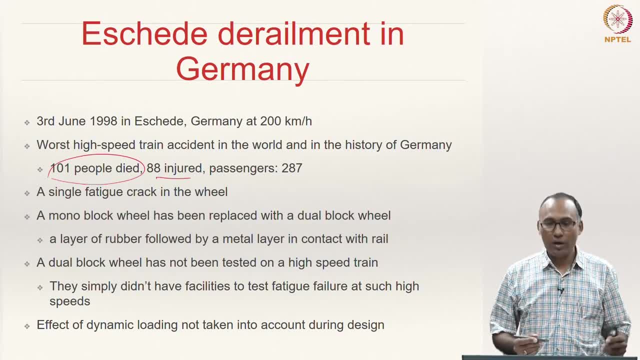 people on board, 88 people injured in a train carrying about 287 people. And what was the reason? The reason was there was a single fatigue crack in the wheel. there was a single fatigue crack in the wheel, and then that is what led to the catastrophic failure of this particular train. So what? 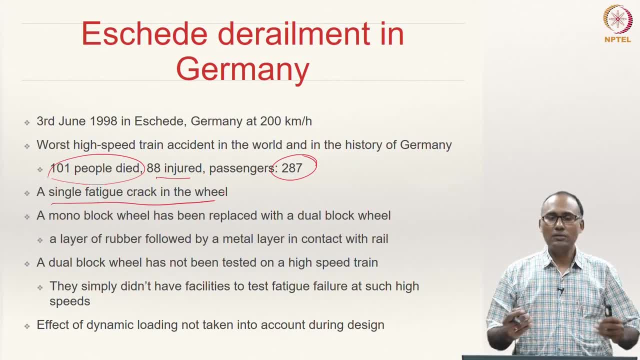 why does this happen? Until then, German Railway, or Deutsche Bahn, was using a monoblock wheel for their rails. and then then, recently, what they have done? Then they have changed this monoblock wheel to a dual block wheel. How does the dual block? 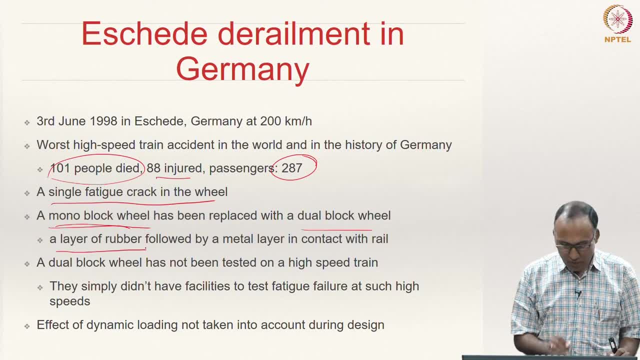 wheel look like They will have a. they had a layer of rubber followed by a metal layer in contact with the rail. So you have first layer of first layer will be metal and below that we will have a rubber layer and then again you will have a rail block. So in order to enhance 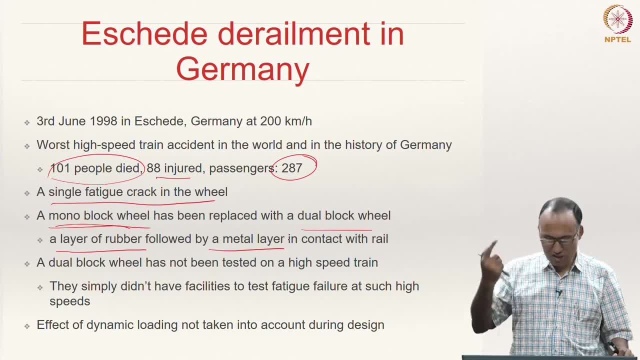 the shock characteristics or vibrations characteristics of the rail, That So just sort of that. or passenger, in order to enhance the passenger comfort, they have done something like that, a design change into their wheels. However, when they have done this design modification, the dual block wheel has not been tested on high speed train. the first thing, The reason: 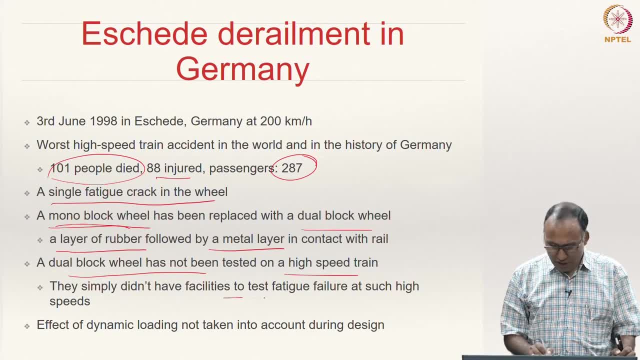 for that is that they simply, at that time, they did not have facility to test fatigue failure at such high speeds, And so they did not have means of what are the reasons? under which circumstances under which it could actually fail, And, while designing, they have not taken into account of dynamic loading during the design of this dual block wheel. 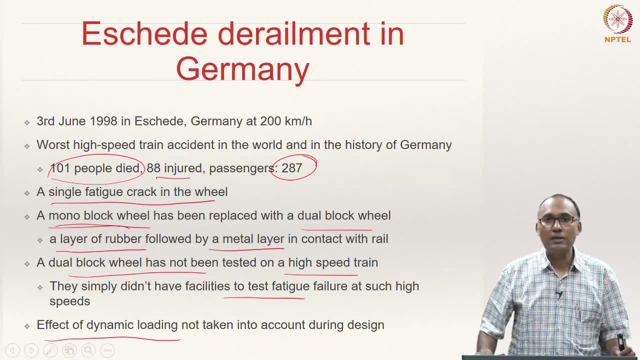 And that led to the failure at the dual block section, that the intersection between the two, So the two, has been added in order that the two end canción son entry points were not stabilurized, So the two end condensers were actually pulled from theirurettes, and that 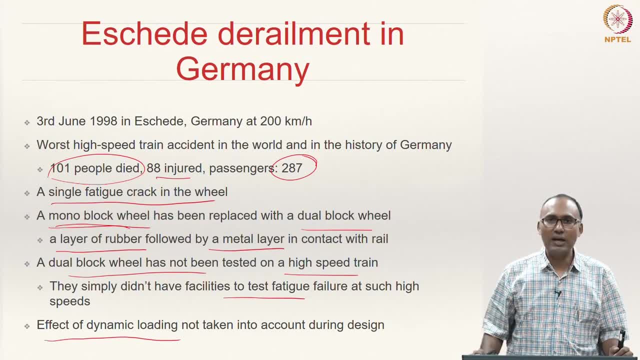 would broken condition. And then what happened is one of the condition of a train. grâce, thank to the protection, It was failed and, however, that construction work was made And based on these這樣 there was a proper specification for the one end serpent and 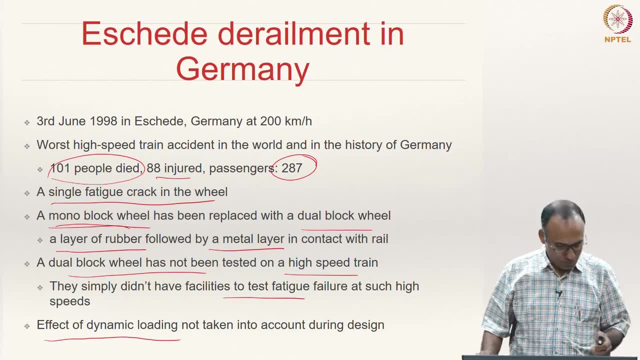 hit the bridge and that led to a catastrophic failure. So all these, basically, are due to as we. the point of discussing these accidents is to actually give you an understanding of the impact of neglecting the dynamic nature of the loads in on machine components and 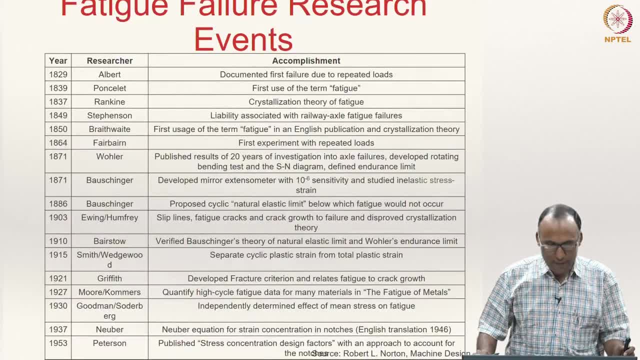 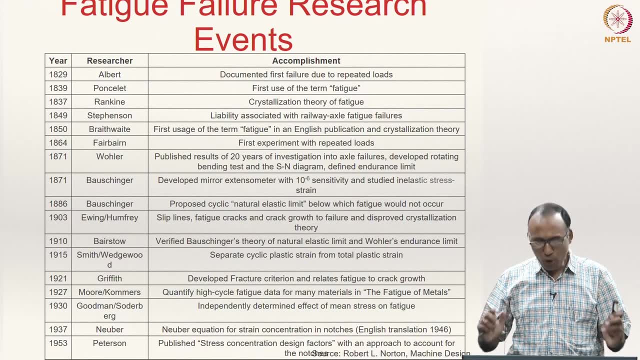 that can actually lead to severe consequences. So there is. this table gives you a an overview of fatigue failure research events in the literature around the world. right? So the first ever failure due to repeated loads was reported in 1829, right? And then 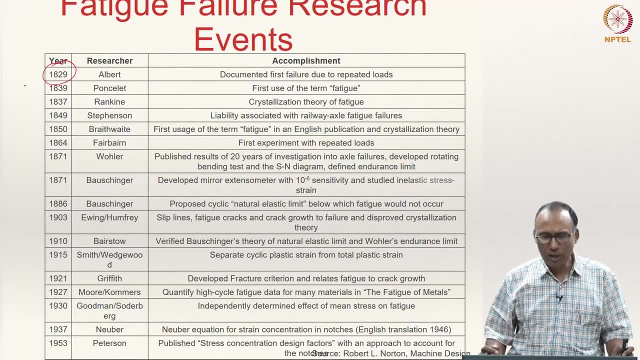 Then several people- Ponkley, Rankine and other people- have spent some time on the first ever usage of the term fatigue in English fatigue was used by Ponkley in 1830s. And then people developed different theories. initially there was a theory called crystallization. 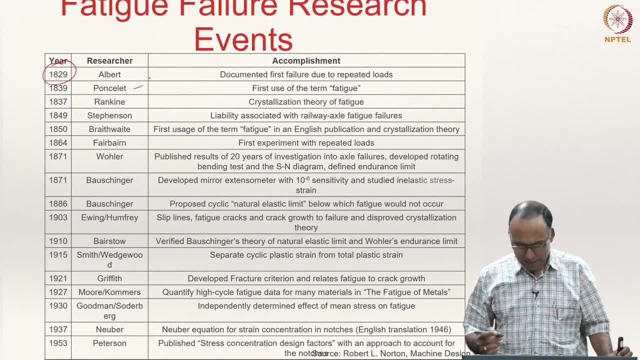 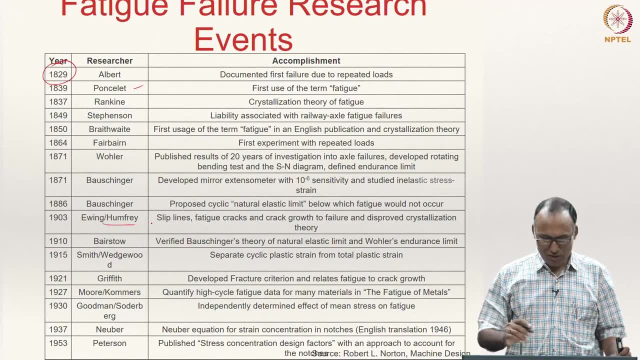 theory for fatigue failure and which was later disproved by Ewing and Humphrey, and saying that the fatigue failure happens due to a set of events like slip lines, fatigue cracks and crack growth, which was actually capable of disproving the crystallization theory hypothesized. 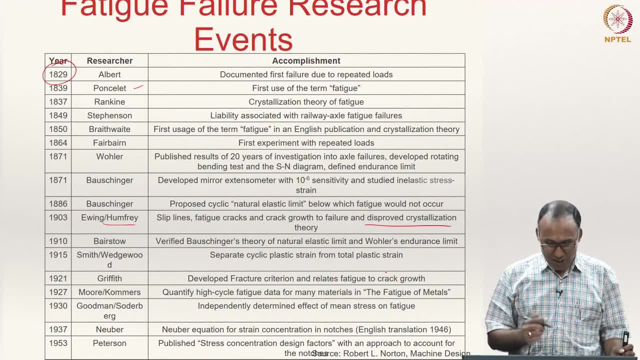 by Rankine and others before that, And the first, probably the most important event in the fatigue failure research happened around 1830s, 1830s, 1830s, 1830s, 1830s, 1830s. 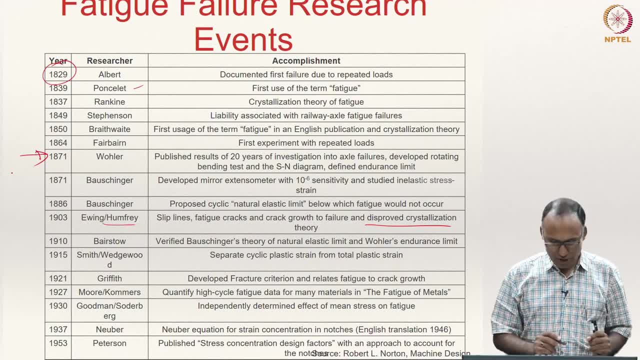 1830s And this time when August Wueler from Germany has published the results of his 20 years of investigation into axial failures And he also has developed a special test called rotating beam bending test, and he is the one who actually given us the concept of S and diagram and defined something called endurance. 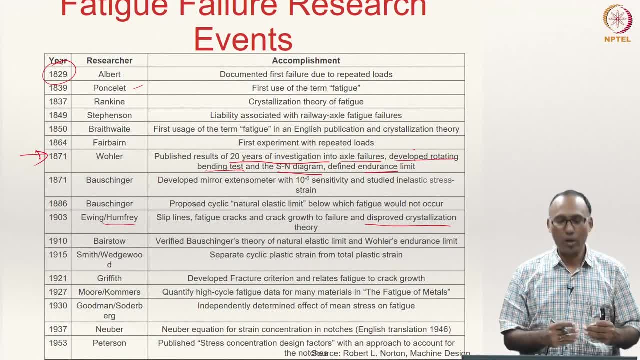 limit. So this is probably 1871, is probably one of the most important years for the researchers of fatigue failure. So So the understanding of fatigue failure actually went to a different level once the Wheeler's 20 years of results are published, And then until the introduction of the fracture mechanics. 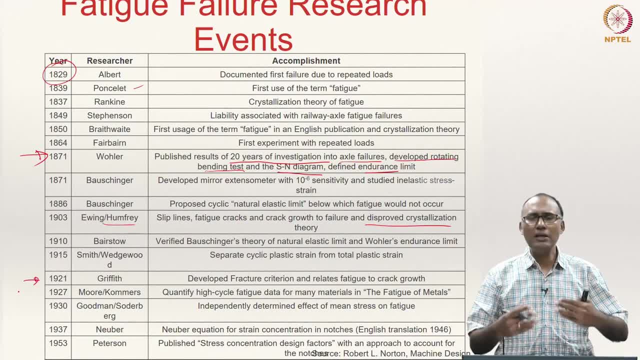 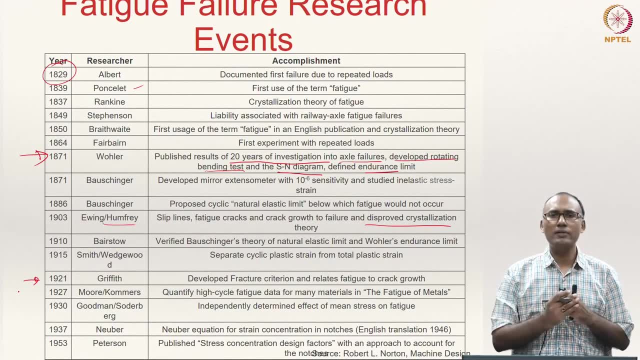 formally by Griffith. there were several theories that were developed, but the Griffiths theory on fracture mechanics really pushed forward the understanding of failure of materials under repeated loading or fatigue loading. And then people like Goodman, Neuber and Soderbergh and Peterson- these people have pushed the field much further. And then today, 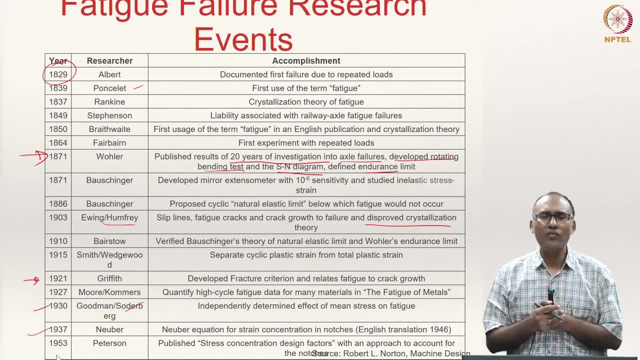 we can say that we have a reasonable, good understanding of fatigue failure, primarily in metals or crystallization materials, to a reasonable extent. So that is why we are able to design structures such that they can withstand the known dynamic loads to certain extent with reasonable factors. 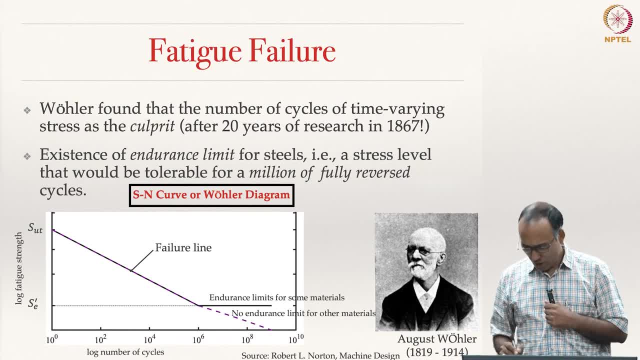 of safety. So this is Auguste Wheeler. So he is the one who actually published first results on a detailed results of his work that he carried out over 20 years. So So he found that what is his seminal contribution? His seminal contribution was that he found that 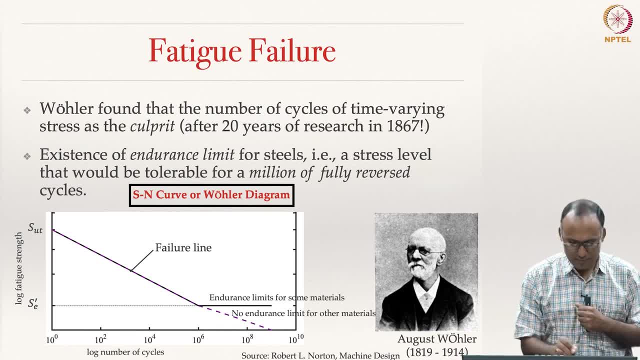 the number of cycles of time varying stress is the culprite for the fatigue failure. The number of cycles of time varying stress is the reason for fatigue failure, And he also has shown the existence of something called endurance limit for steels. That means what? do you mean by endurance limit? An endurance limit is the stress level For any particular material. this stress outside the supply chain, this pressure is energy continuous. This diameter is duration. duration, For example, if we look at the release time limit of brakes and Enterop zustantial. 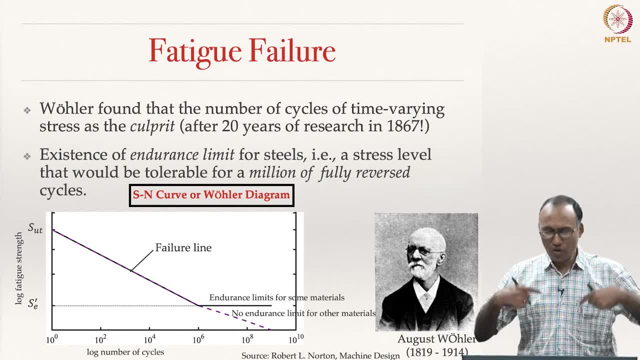 level that would be tolerable for a millions of, for a million of fully reversed cycles. We will talk about what do we mean by fully reversed cycle. but what he is saying is, if your stress level is below certain value, then you can say that the material will withstand. 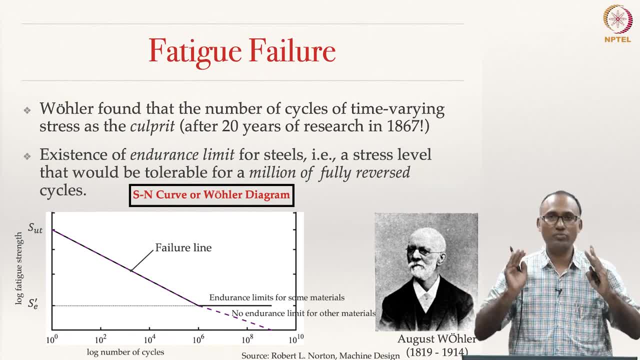 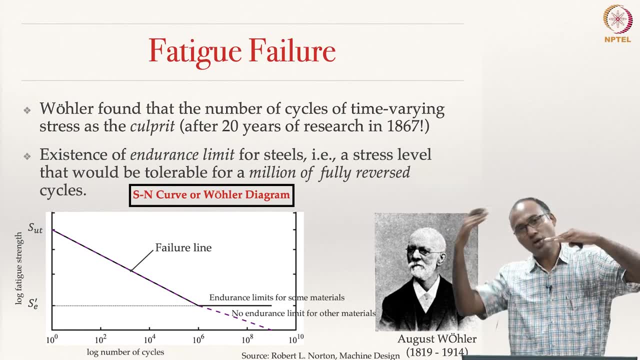 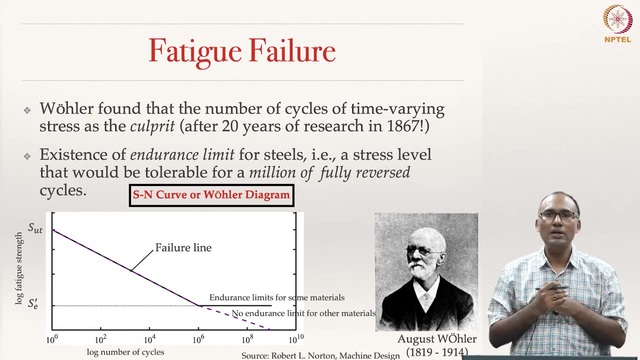 1 million cycles of that, if the stress level is below some value, And that value, below which you will have life beyond 1 million cycles, is called endurance limit And sometimes people in some text books they also use it as endurance strength of the material And 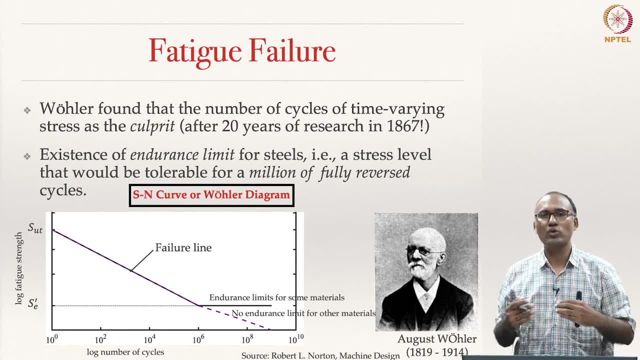 this is typical for steels. primarily his work was on rail axles and hence he gave this conclusively for steels. This is the diagram here. shown here is actually the schematic of SN diagram. What do we mean by SN diagram? S is your stress amplitude. we will talk about it. what do we? 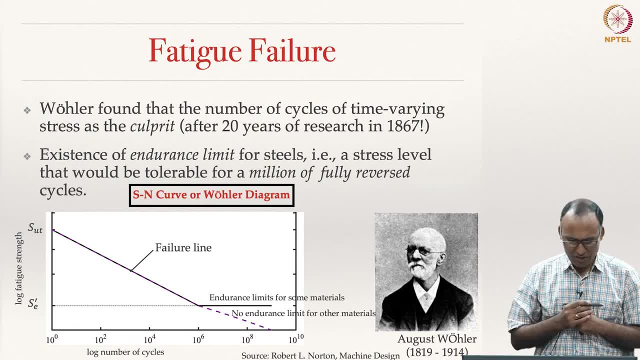 mean by stress amplitude and by and the X axis, you have number of cycles, And please note that here you see a straight line, but it is on a log scale, right, it is a log, log scale and hence it is not really a straight line. 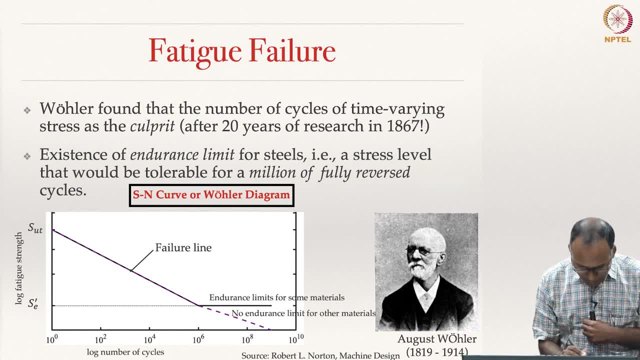 It is a power log and then you see that, let us say 10 power 0, that means 1 cycle. when you have 1 cycle, The fracture, when we are talking about fatigue, we are actually talking about crack propagation. that means we are actually talking about breakage And hence we are not, we cannot talk about. 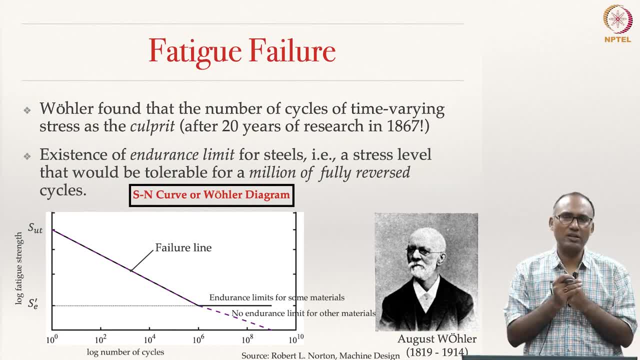 yield strength of the material anymore. we should be talking about ultimate strength of the material, right. So the ultimate strength, alright. So when you have 1 cycle, that means there is only 1 cycle, that means there is no repeated loading, And hence you can actually 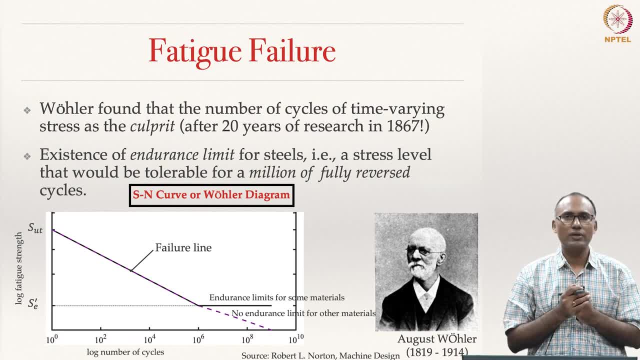 think that situation as the case of static loading, right And now. so that means the material fails at SUT and now if you have your stress amplitude somewhere in between, then you can say that the failure happens at somewhere. like it is 100 and 1000, say, may be something. 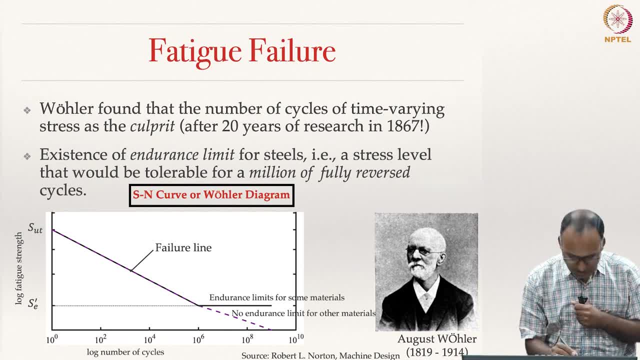 like 9000, 900 cycles. So here let us say, this is 900 cycles, So the failure happens. So the failure happens of 900 cycles. that means what at this stress amplitude S a, I can use my component for 900 cycles. after 900 cycles it will break. So that is so that. 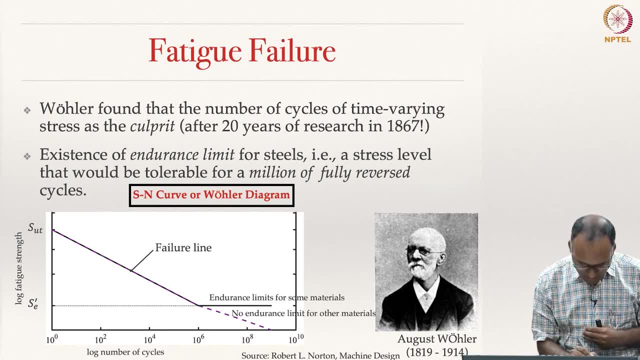 means this is what you call life and this is what is called stress. So S n diagram is nothing but stress, life diagram, or it is also called Uhler diagram And, as we have discussed, endurance limit, that that is described by S e dash.